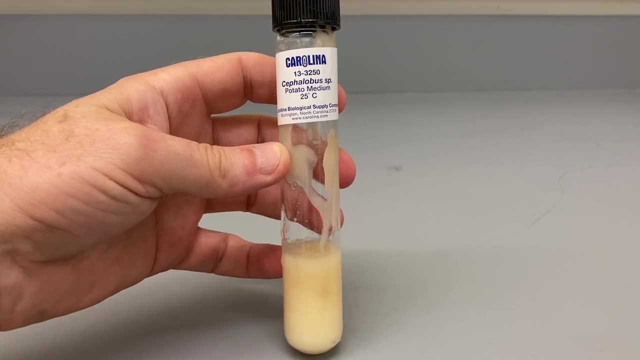 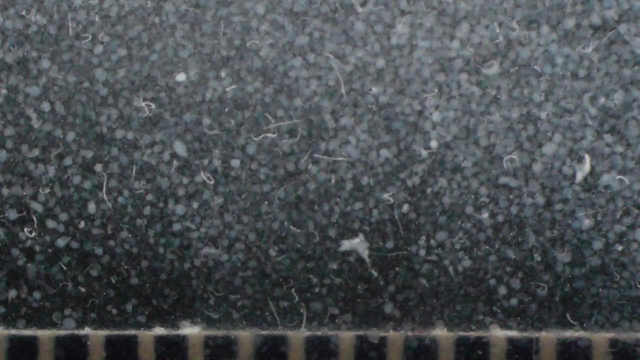 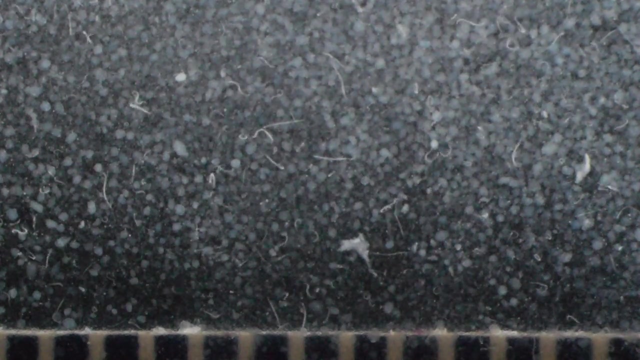 These are being raised on what is basically rotting mashed potatoes, where they are eating the bacteria growing on the potato bits. Here are a few. in diluted medium, The spherical objects are little bits of potato. Nematodes almost always wriggle in this particular distinctive way so that even if you see them at low magnification you can immediately identify them as nematodes. 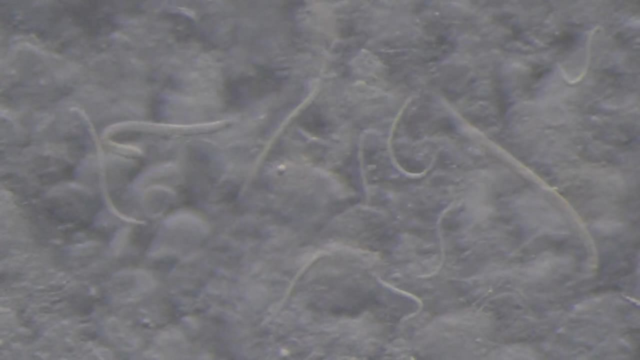 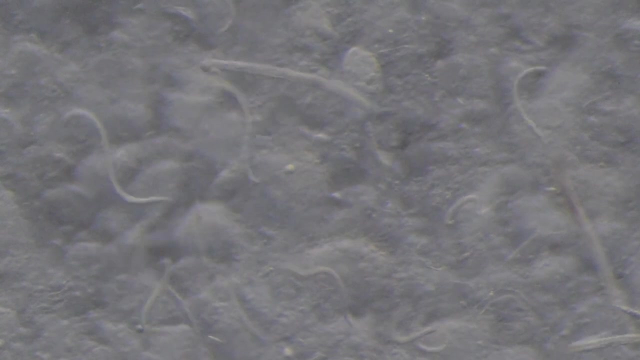 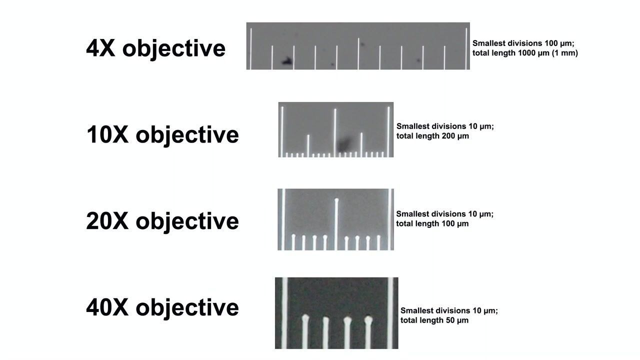 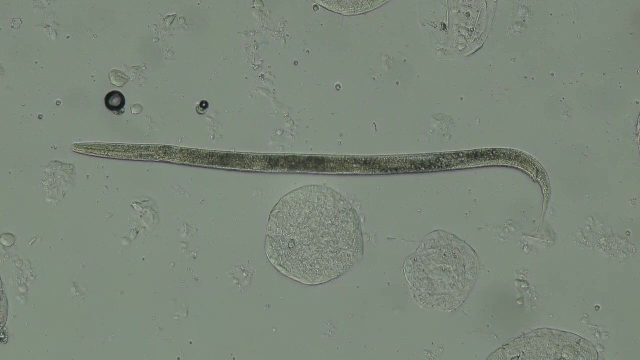 They're also a very large group of animals. To see their anatomy a little better, I killed a few individuals by heating them up. Here's a male inside view. Males of most species of nematodes typically have a bent or hooked posterior end. 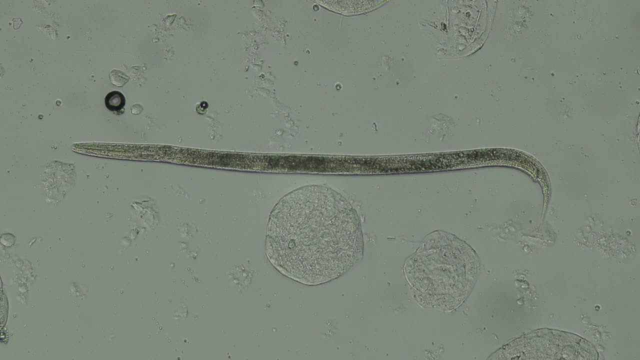 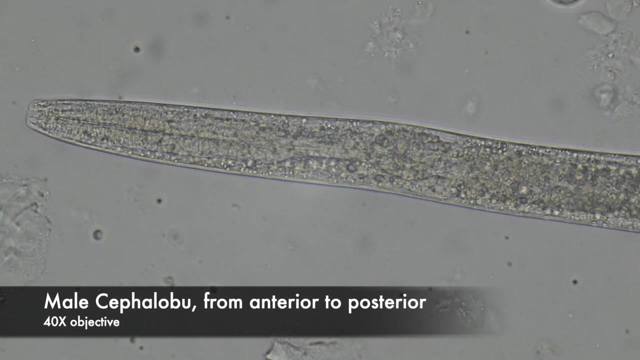 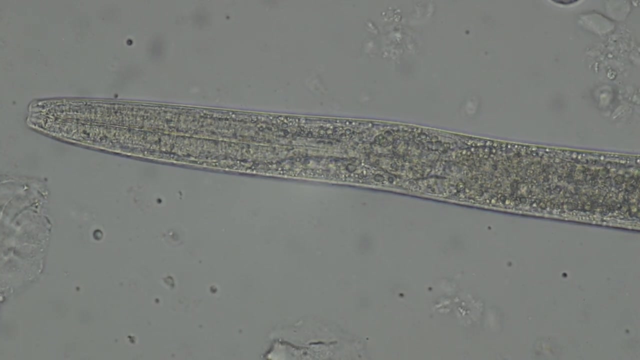 They use that bend to grasp females when they're mating. The very anterior end is usually pretty blunt-ended. In this one you can faintly see the pharynx which has two concentrations of muscles or bulbs. That pharynx is used to suck in bacteria-rich fluids around them. That's what they're. 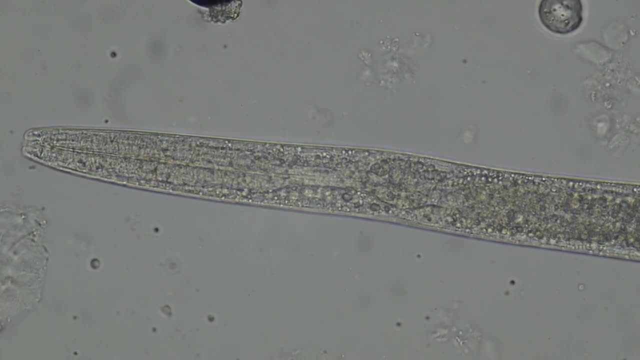 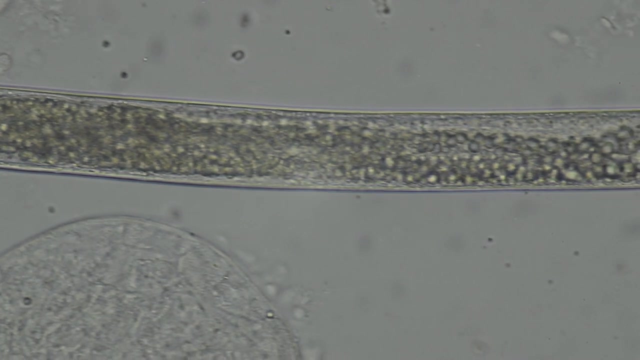 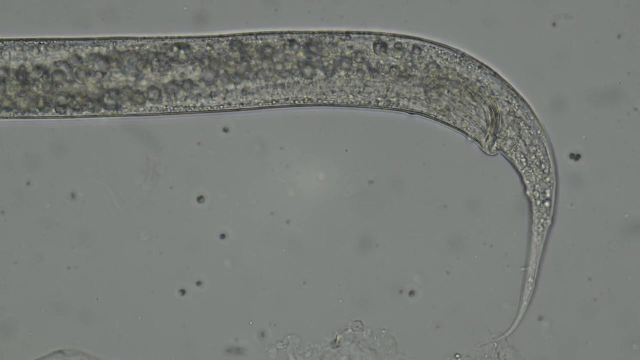 feeding on. Near the posterior end you can see a little bulge. That's the cloaca, out of which the anus and the male gonopore open. Males have a set of copulatory spicules that can be extended out of that opening. Here's another male with a. 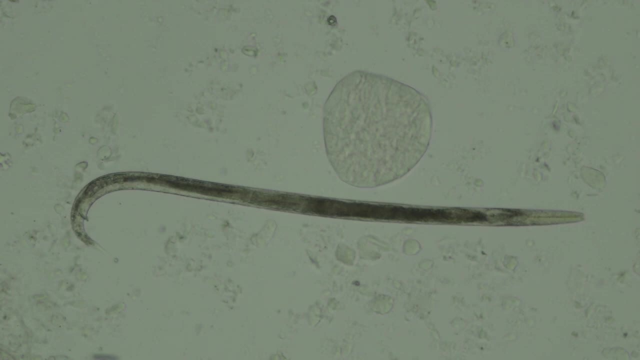 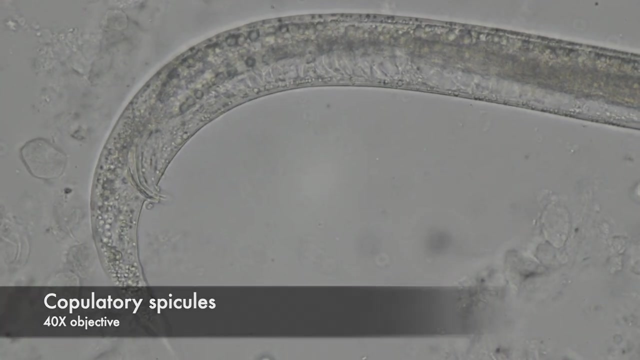 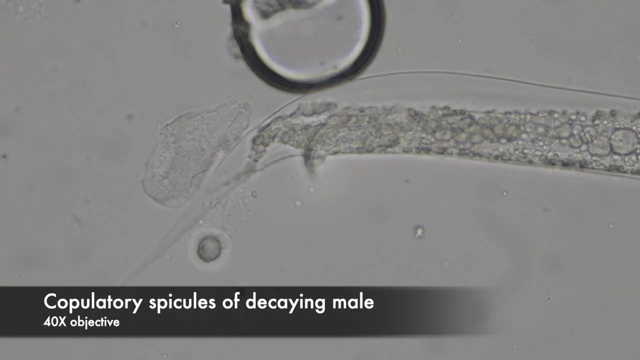 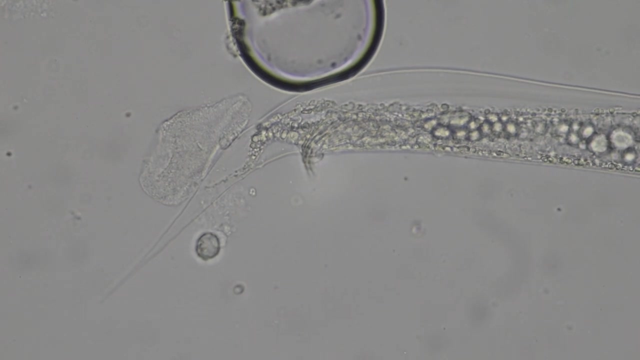 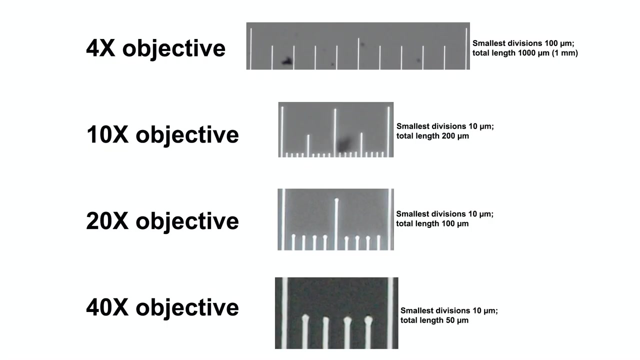 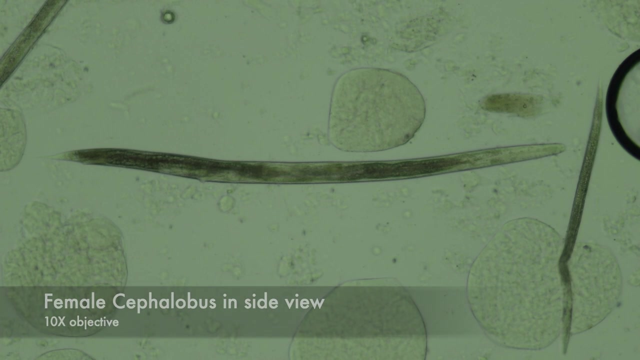 slightly more obvious set of copulatory spicules. They use those to help transfer sperm to females when mating you. And here's a dead individual whose copulatory spicules are sticking out a little bit and are particularly easy to see. Females don't have that hook in the posterior end and they also have 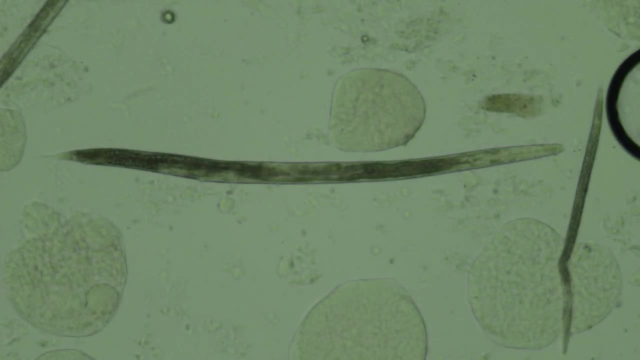 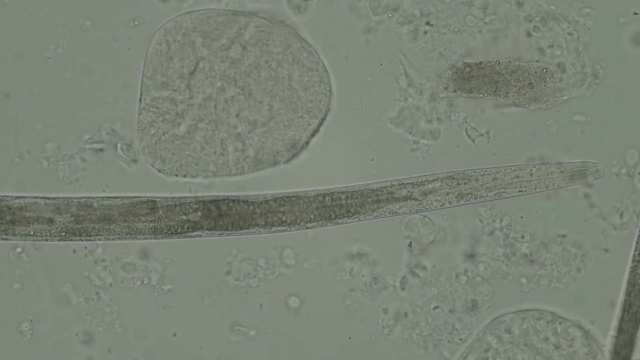 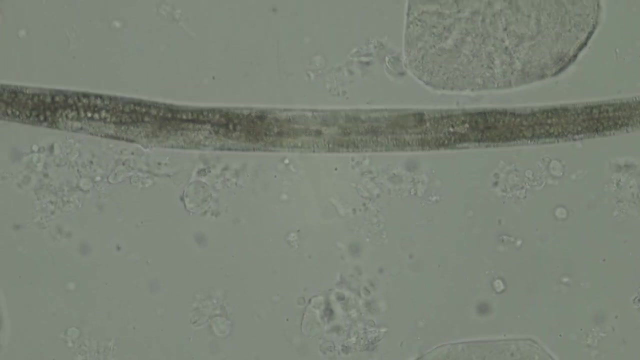 separate openings for the anus and the gonopore. This female's anterior end is on the right, posterior to the left, One female slowly keepsшеaring straight and two in their own wait and guess where Patreon paid for to have them. Do you want to use more gloating? 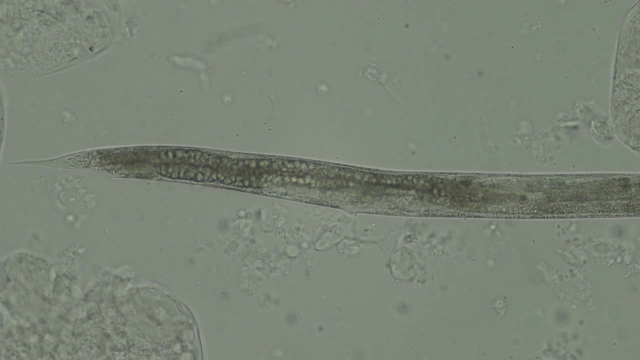 Hence Sorry, Gam, trekking on top of my muscles. double hand experiment. In this female's posterior half you can see two bumps. Those are circles on the. The posterior one is the anus. The one closer to the middle of the body is the female gonopore. 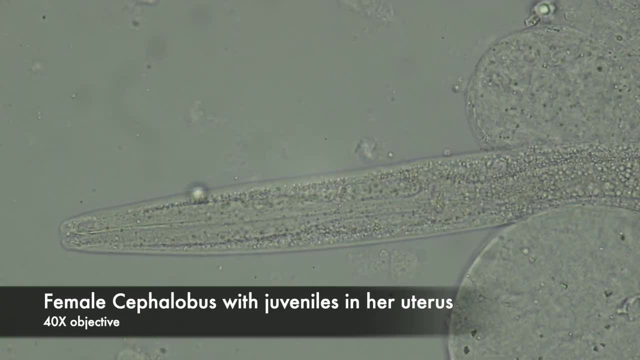 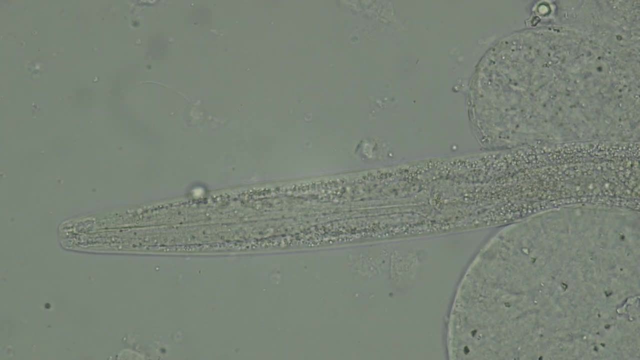 In cephalobus, sperm enter the female gonopora mating and embryos develop to the first larval or juvenile stage inside the mother. This female, who has a really nice pharynx, is carrying three or four young worms inside of her. 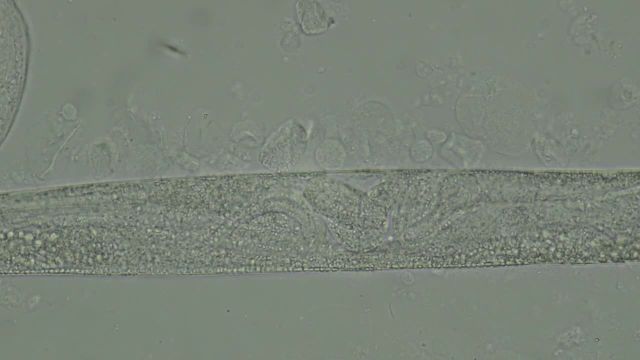 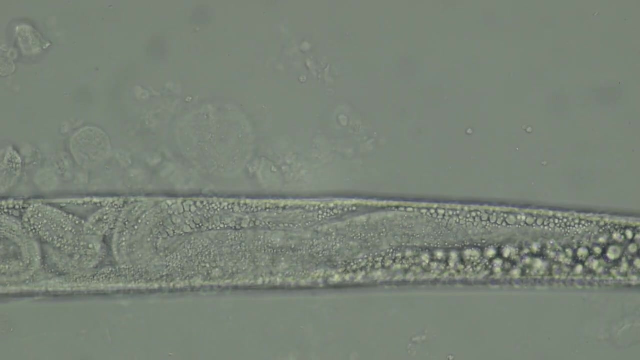 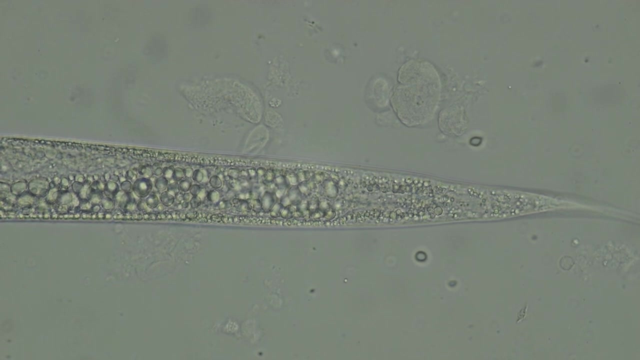 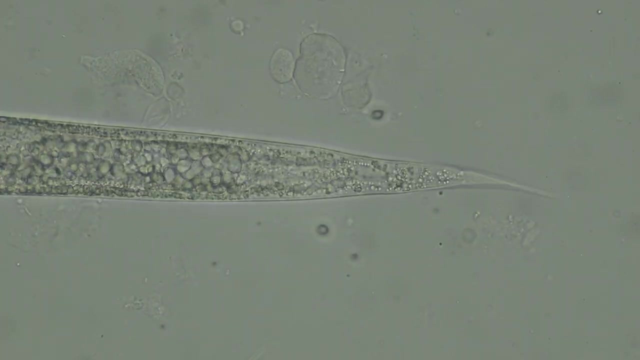 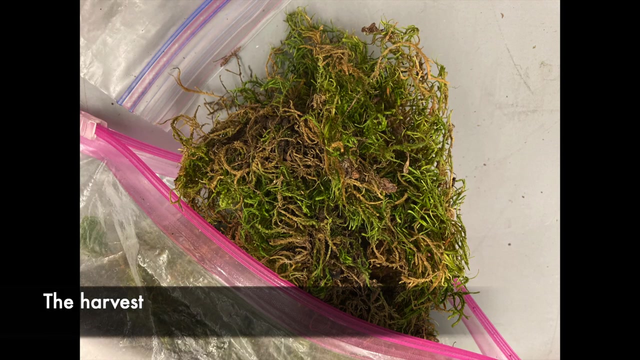 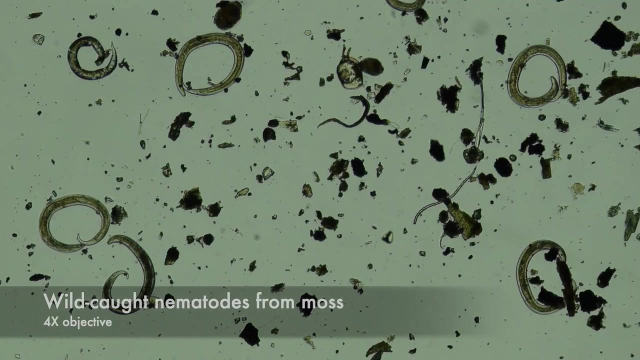 This female is not in side view, though, so we cannot see her gonopore or anus. I also caught some wild nematodes in moss my father collected for me in Sonoma County. After soaking it in spring water, I found lots of deloid rotifers and also lots of these coiled anhydrobiotic nematodes. 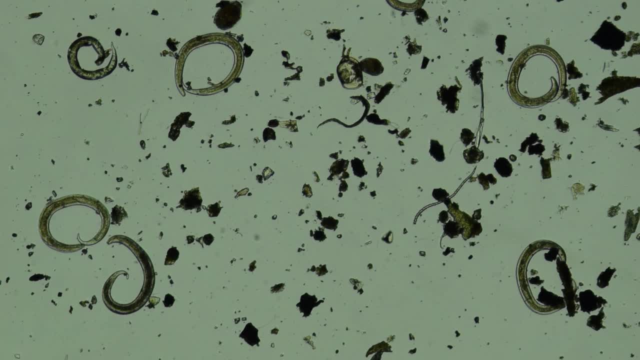 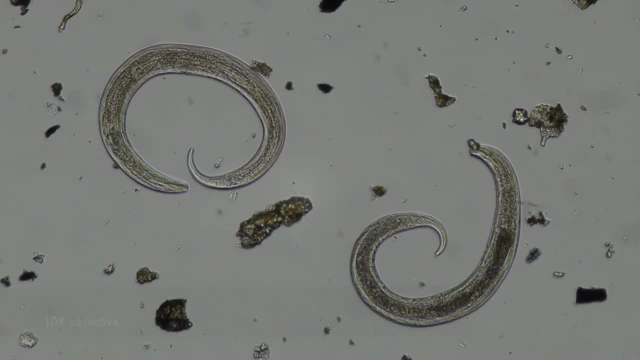 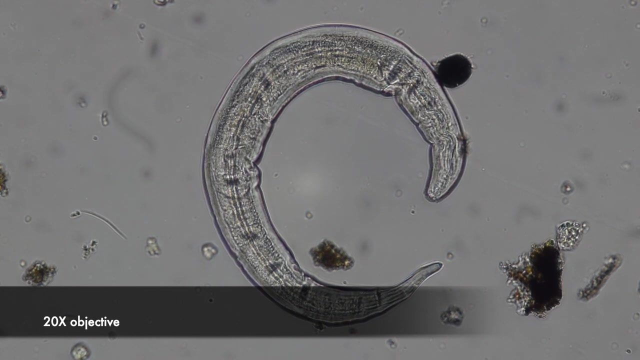 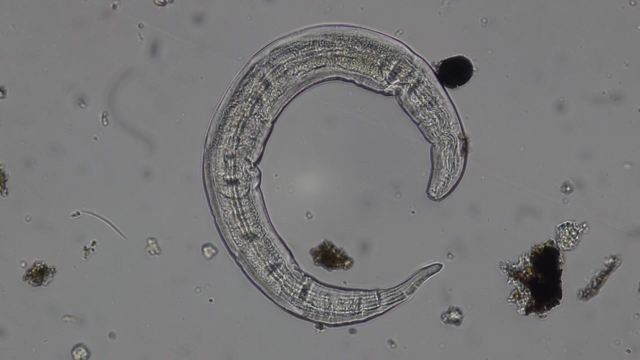 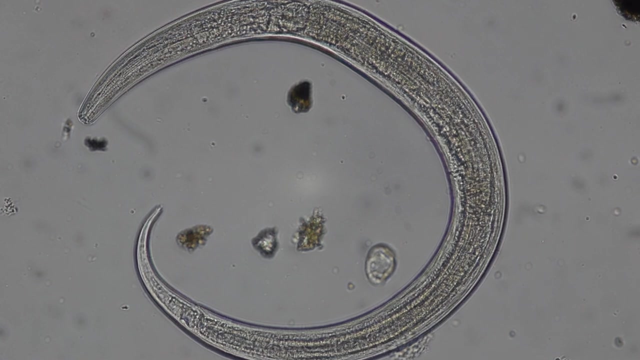 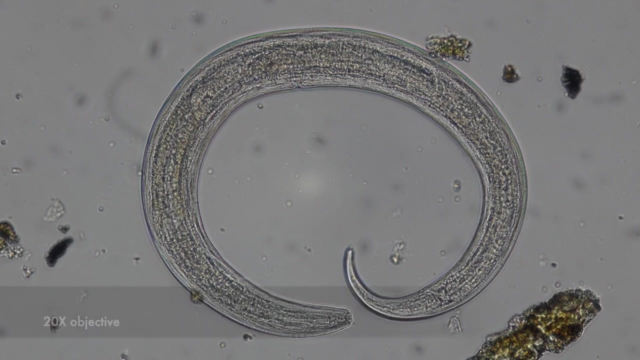 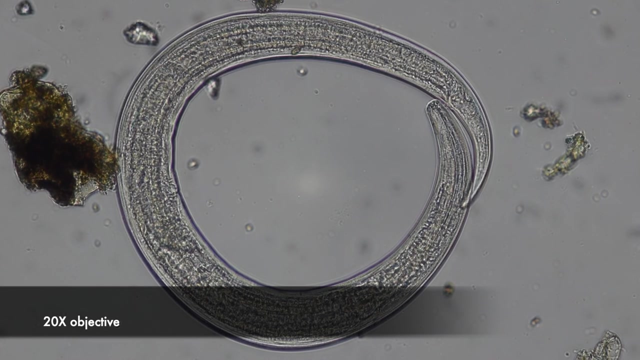 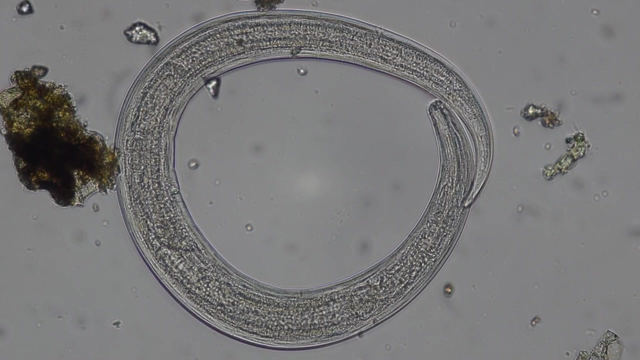 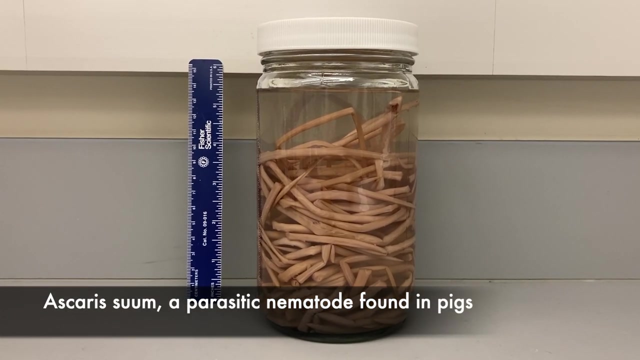 I'm sure that these are alive, but they did not become active in the two or so hours that I watched them. To be continued, There are thousands of species of parasitic nematodes. Here's a nice large one, Ascaris sum, which, as an adult, lives in the intestines of pigs. 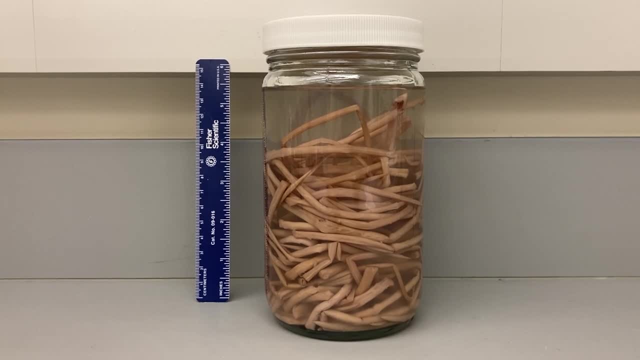 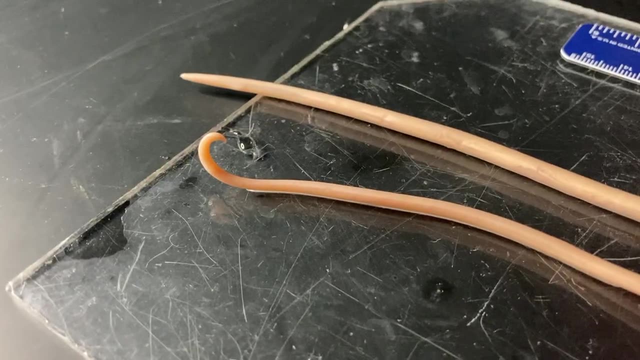 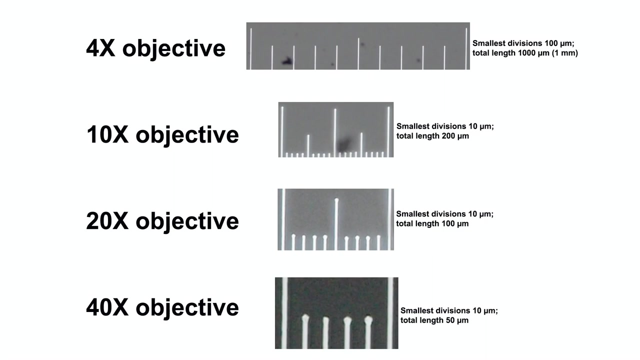 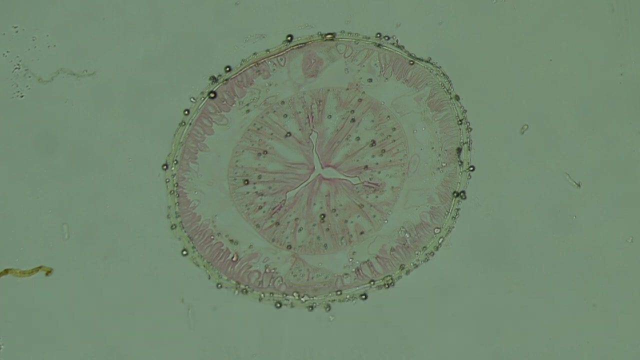 This jar contains maybe 50 individuals. Here are a male and female individual. The male has that typical hooked posterior end And here's a cross section through an Ascaris made at the level of the pharynx. Ignore the little air bubbles that are developing in this section, which is really old. 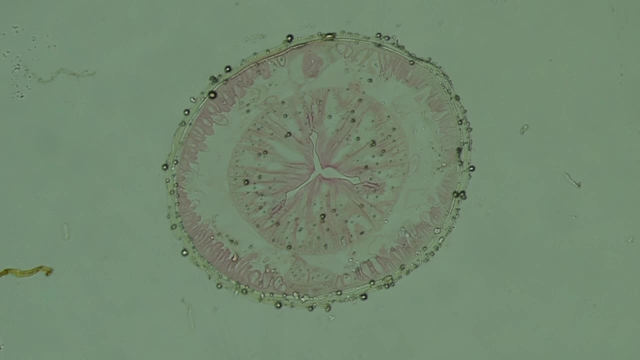 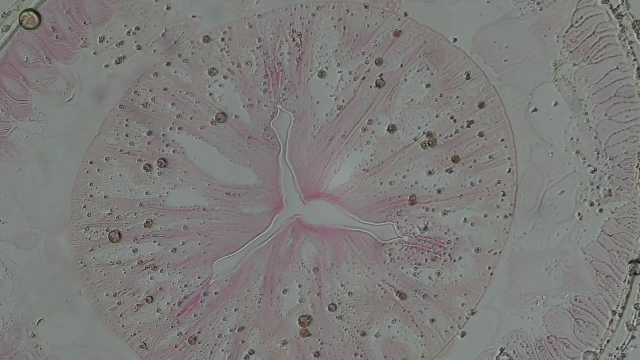 But in this section you can see great cuticle, longitudinal muscles in cross section, the dorsal and ventral cords, the pseudocel and of course the huge muscular pharynx- pharynx. Dr Ralph Appie kindly provided me some nice images of another parasitic. 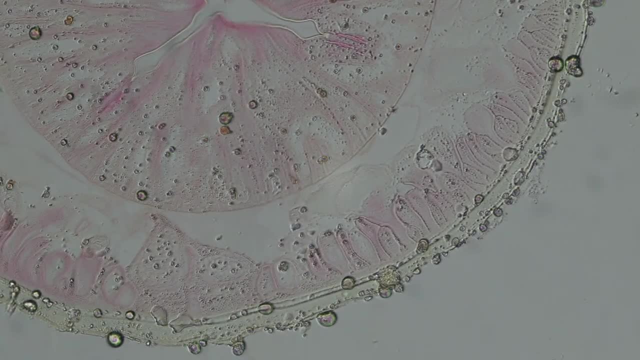 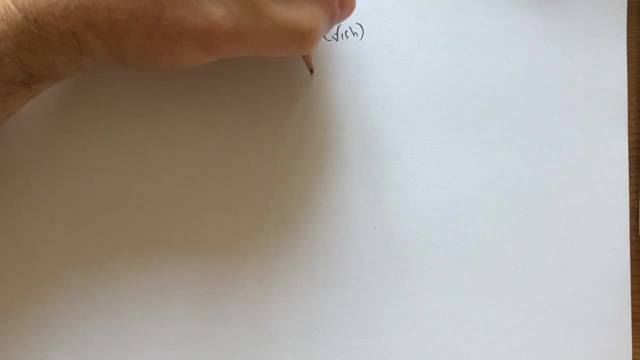 nematode Spirochamelonis pureri through its life cycle. This nematode is common in Southern California, where its final host can be any one of a number of bony fishes, mudsuckers, croakers, top smelt, but others as well- Mated females release. 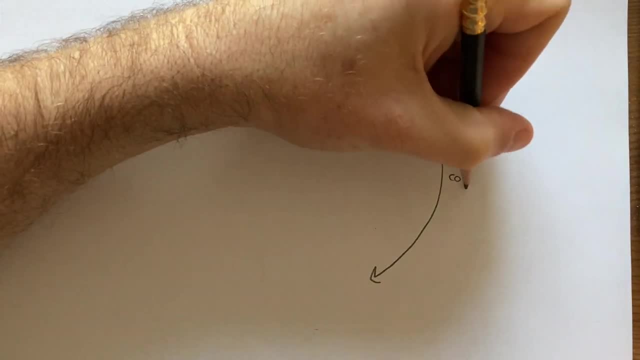 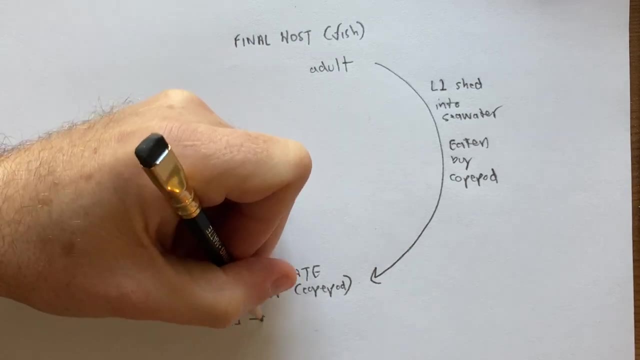 juveniles, which nematode people usually call larvae. Specifically, they release the first juvenile stage, which we can call L1. Copepods then ingest those whole and they continue developing in the copepod. They molt into L2 and L3 in the 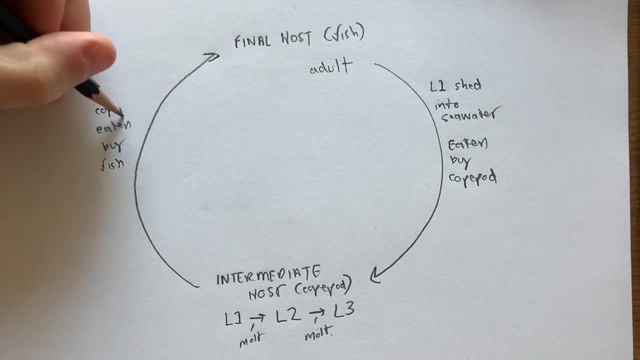 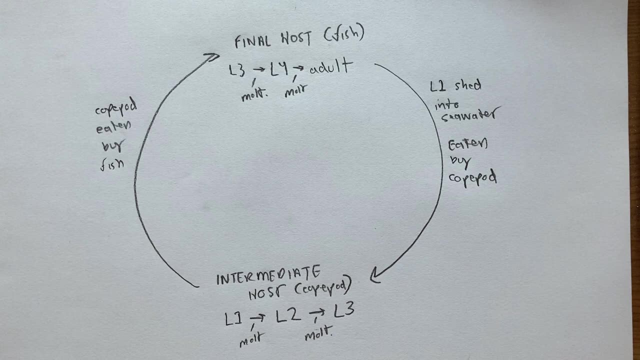 copepod. Then when the copepod gets ingested by a fish, the L3 stage infects the fish In the fish- L3, molts to L4, and L4 to adult. And then the adults mate and the whole business starts all over again. Here are some L1 juveniles or larvae. 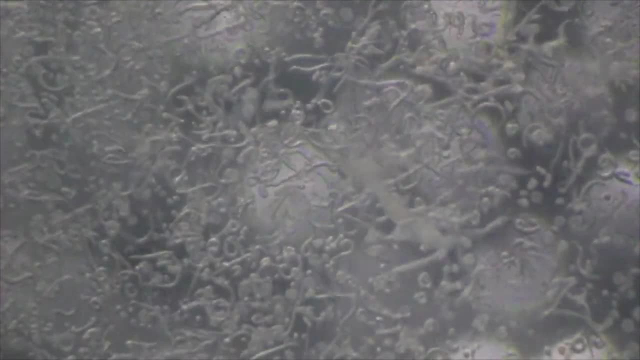 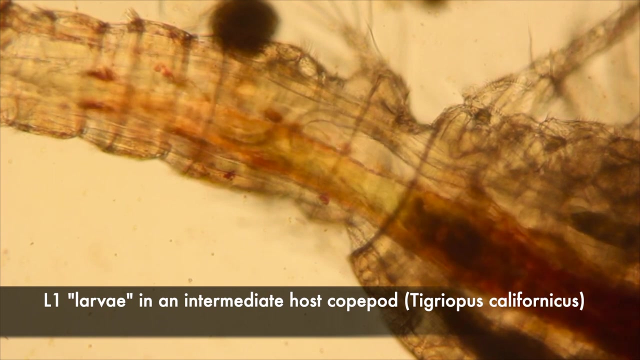 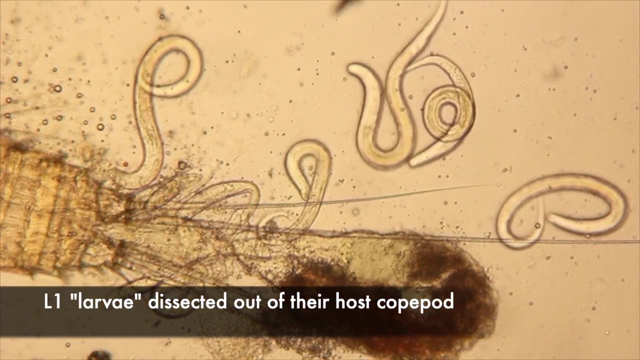 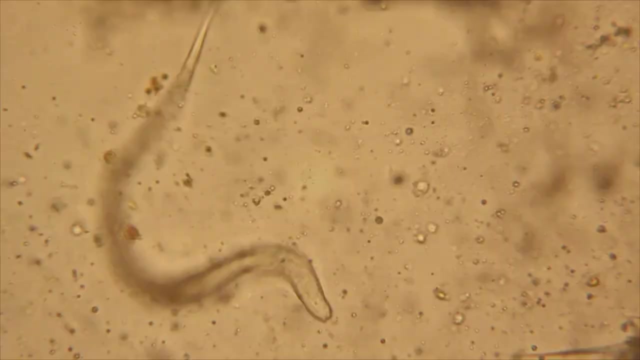 just released from the mother And here are some L1s happily living in their new home, the copepod Tigriopus californicus. Look at that long skinny tail That will change in shape at the molt from L2 to L3.. 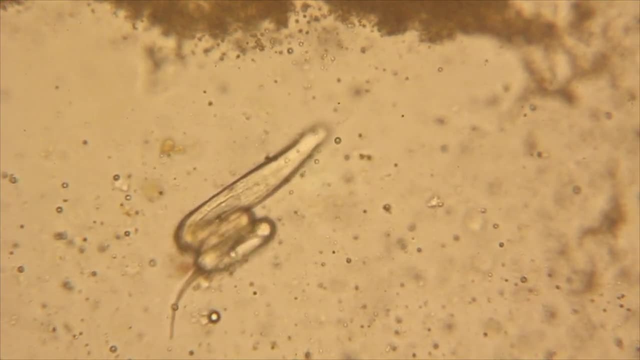 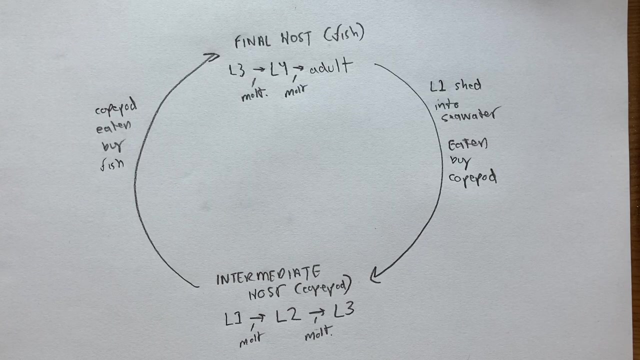 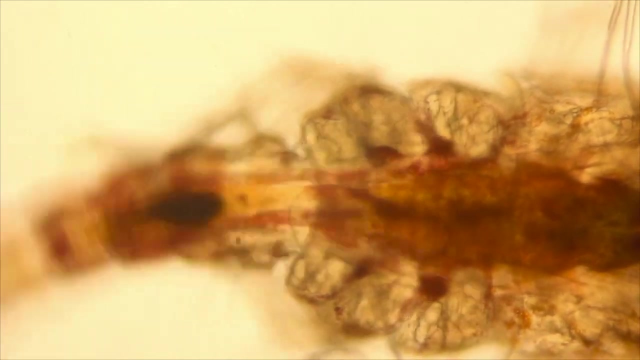 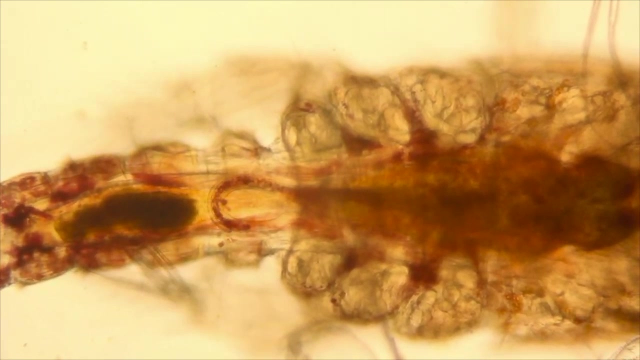 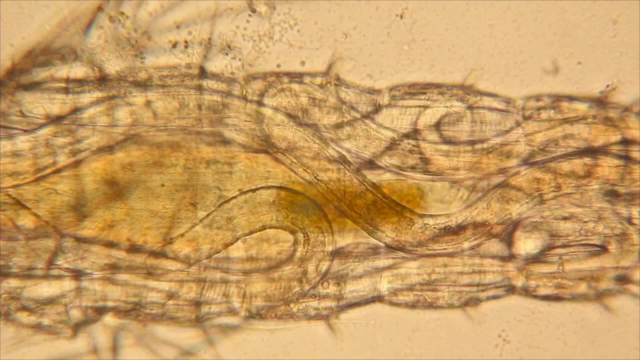 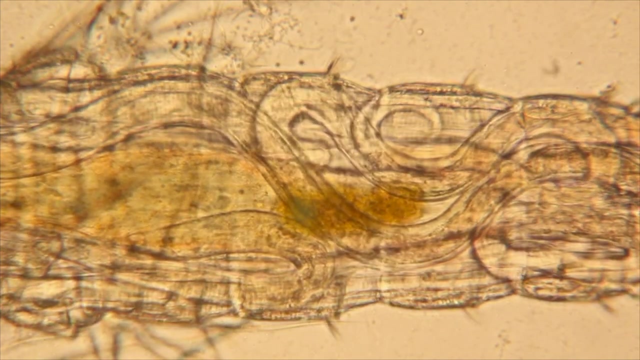 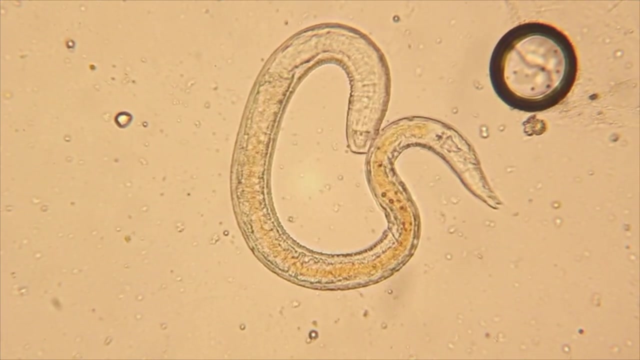 Here are some L2s in the copepod. They're clearly doing some eating in there, as there is something in their guts now and they're larger than L1s, of course I'll engage that N3 guy. Here's an L2 that's just about ready to malt into L3.. You can see the new posterior end is.